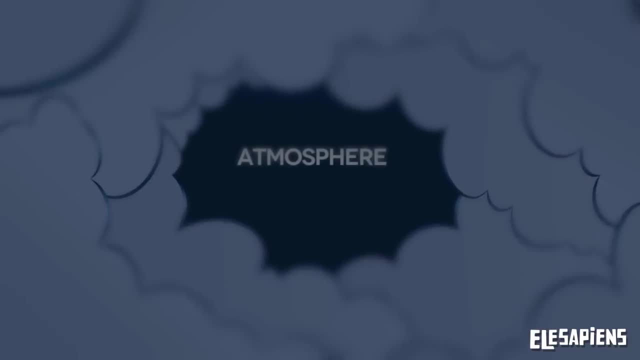 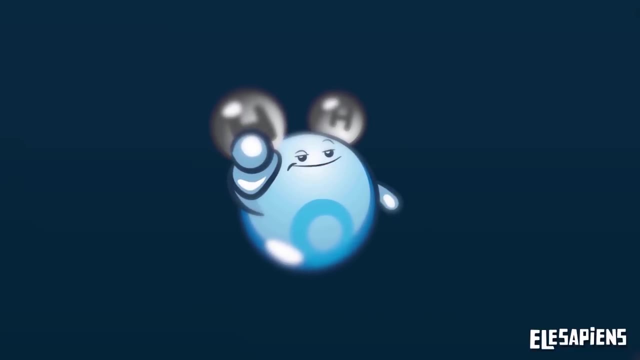 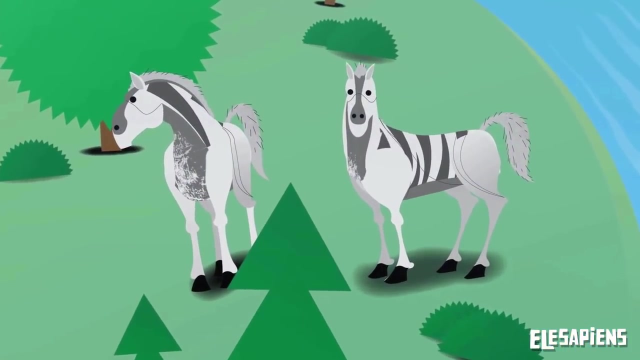 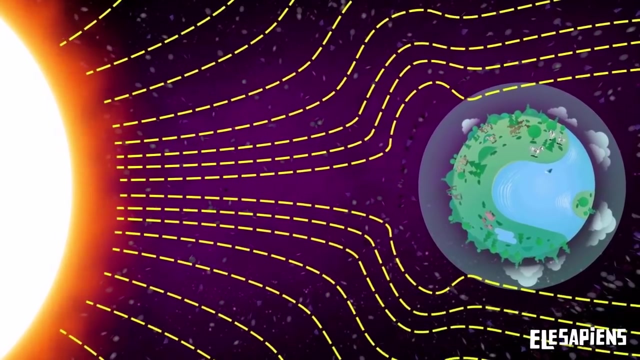 How are clouds and storms formed? The answer is found in the atmosphere. Yes, here in the atmosphere. Atmosphere- Do you know what that is? The atmosphere is a layer of air surrounding the Earth. It allows all living things to breathe, regulates the planet's temperature and protects it from particles and radiation from the sun and from outer space. 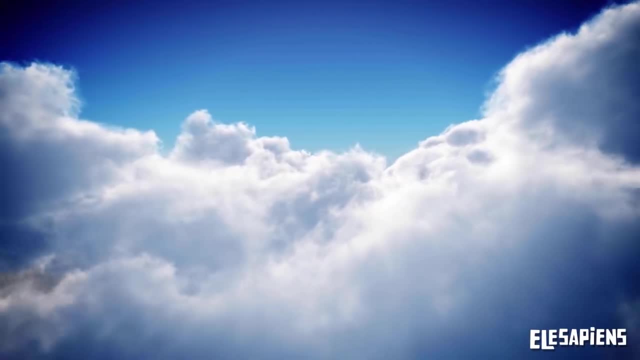 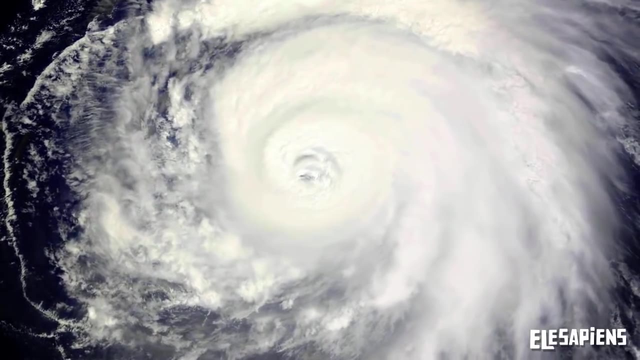 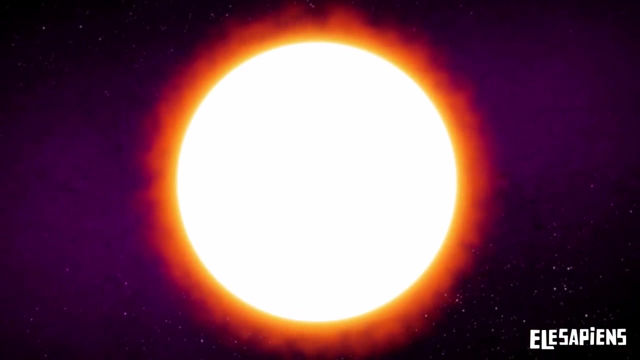 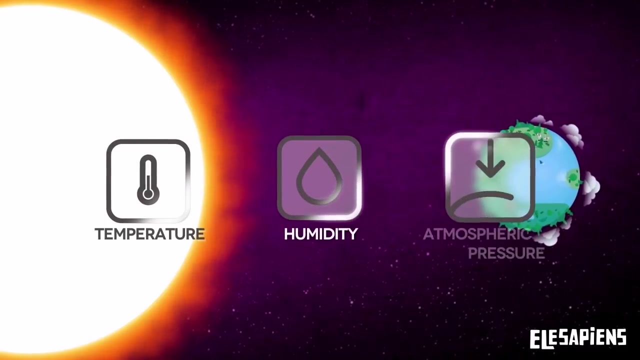 All phenomena that determine weather conditions occur in the atmosphere. Clouds, rain, winds, storms and hurricanes are formed in the atmosphere, But how do they occur? All atmospheric phenomena are originated by the sun. The sun influences all weather elements, such as temperature, humidity and atmospheric pressure. 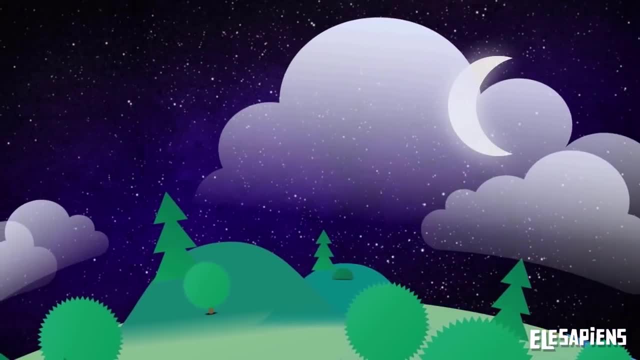 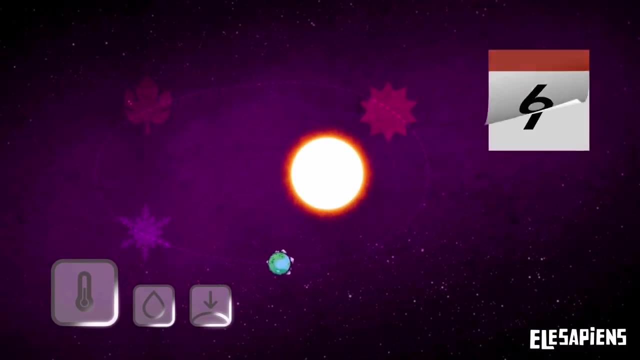 Temperature is the amount of heat or cold in the atmosphere. It changes throughout the day, seasons and regions according to the position of the Earth relative to the sun. Humidity is the amount of water in the atmosphere evaporated by the heat of the sun. 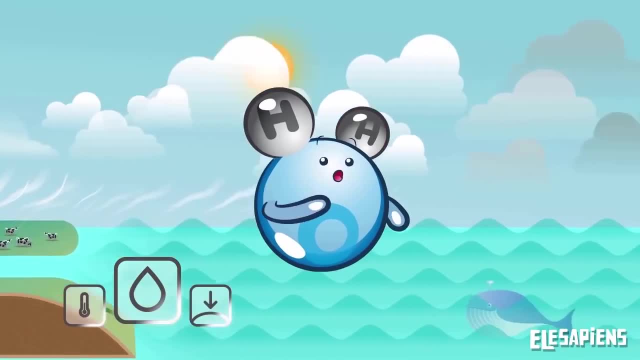 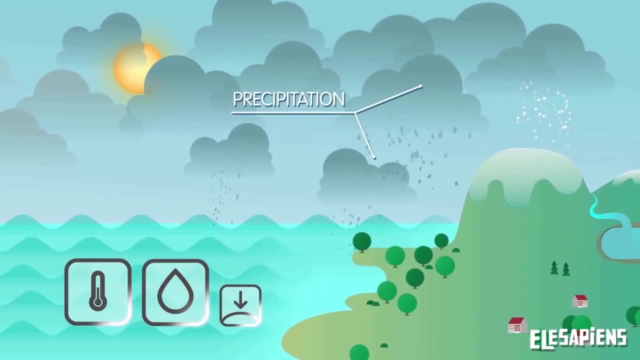 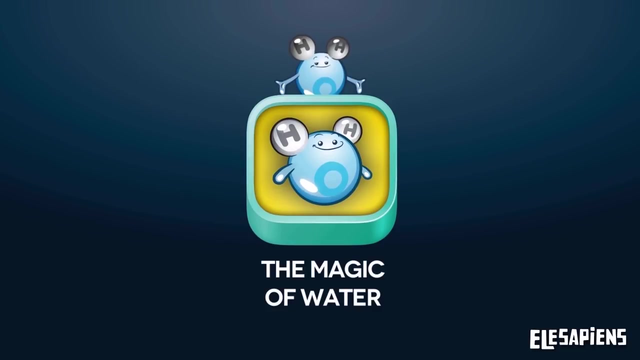 Have you heard of the water cycle? Me me, mine. Humidity and temperature in the atmosphere are responsible for the formation of clouds and rain. I'll tell you more about the water cycle in The Magic of Water. Atmospheric pressure is the weight of air over the Earth's surface. 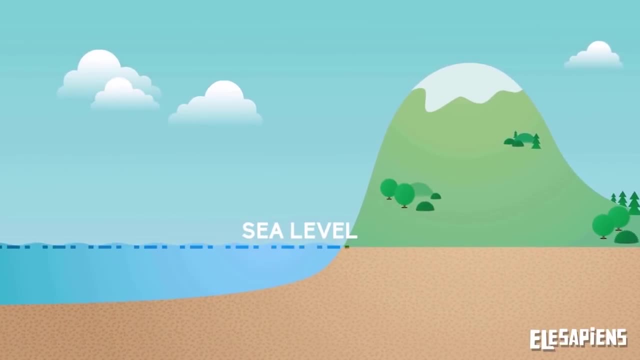 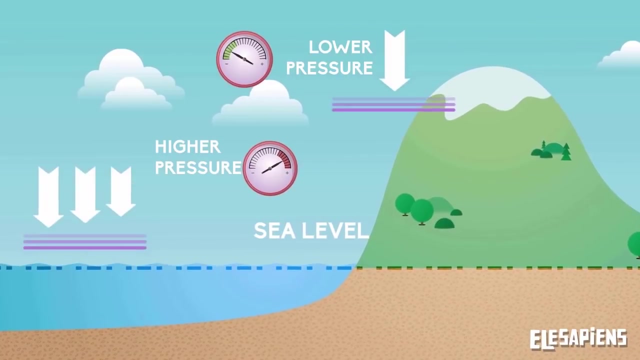 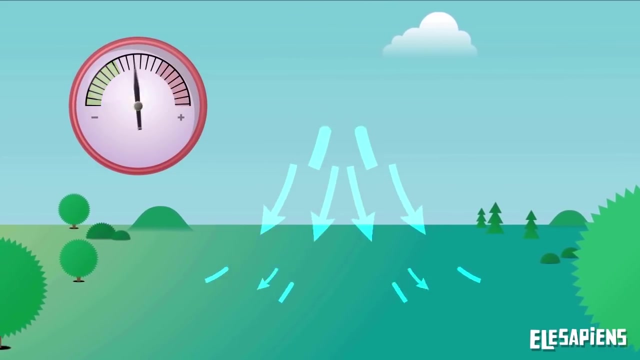 Air has weight. We live at the bottom of an ocean of air. The more air above us, the greater the pressure. Pressure changes with altitude and temperature. Warm air is lightweight and goes up and is replaced by cold air, which is heavier and goes down. 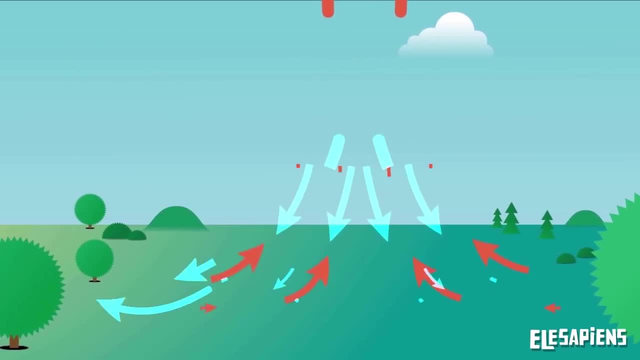 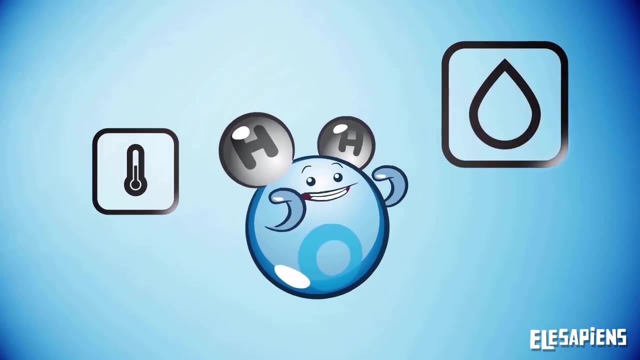 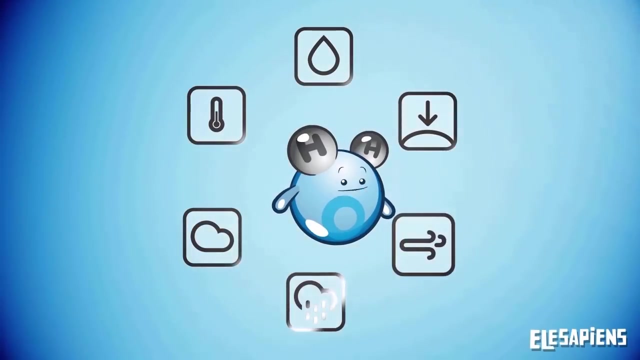 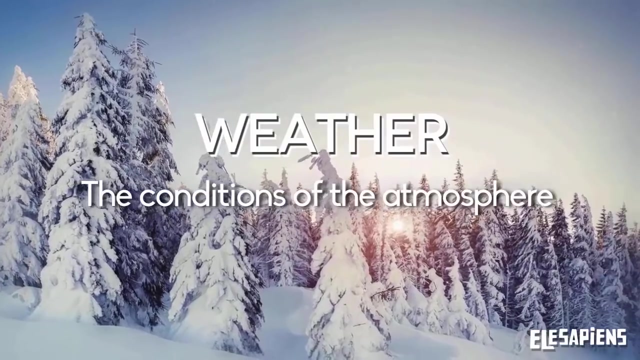 This movement of air masses produces winds. Temperature, humidity and atmospheric pressure are some of the weather elements, although there are more, such as cloud coverage, rainfall and wind. Weather and climate are not the same thing. Weather describes the conditions of the atmosphere at a particular time and place. 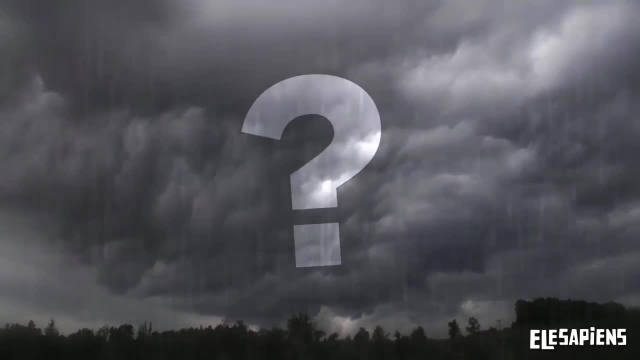 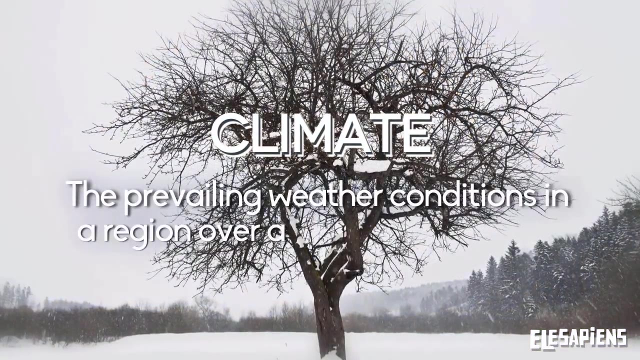 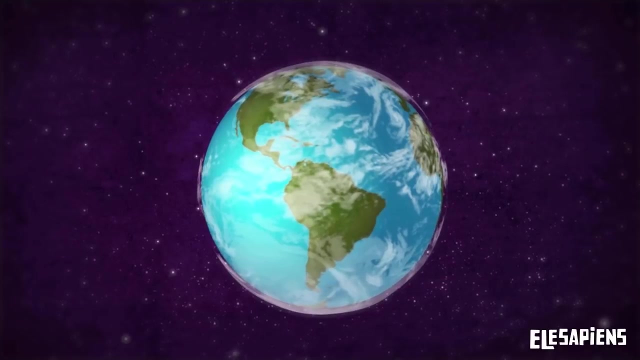 Here and now, the weather is cloudy and rainy. What's the weather like where you live? Climate, however, describes the weather of a region over a longer period of time. The weather and other factors such as landforms, the proximity of the sea and the temperature of the air are all related to climate.